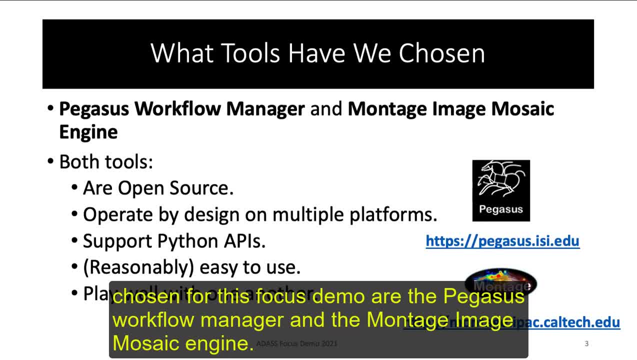 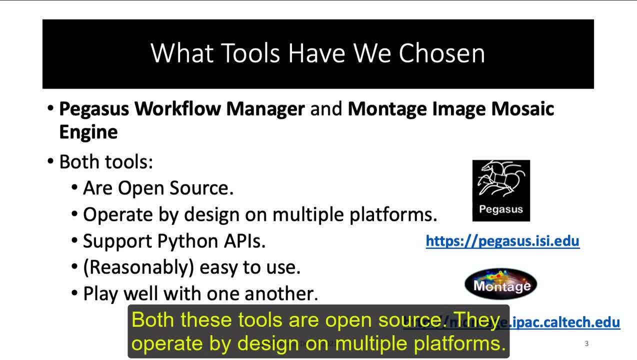 So the two tools that I'm going to talk about today are: the first one is the tools we have chosen for this focus demo are the Pegasus Workflow Manager and the Montage Image Mosaic Engine. Now, both these tools are open-source. they operate. 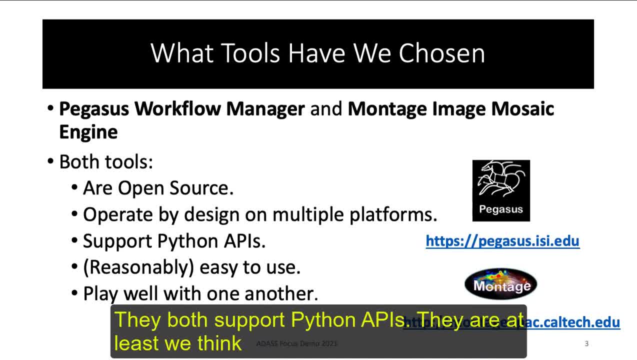 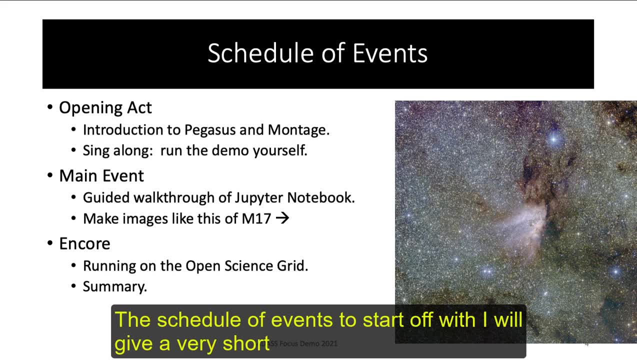 by design on multiple platforms. they both support Python APIs. they are, at least we think, reasonably easy to use and they do play well with one another. So a schedule of events To start off with. I will give a very short introduction to. 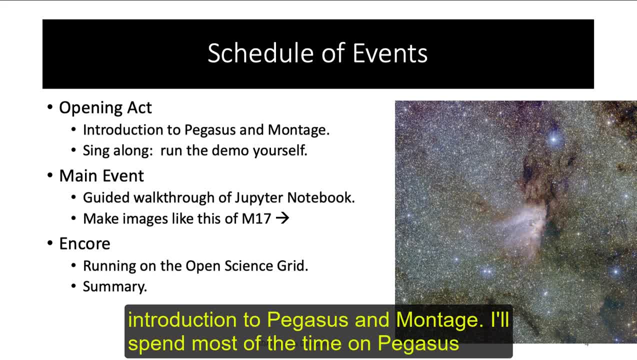 Pegasus and Montage. I'll spend most of the time on Pegasus, since people at ADAS are probably less familiar with it than Montage, which I've spoken about probably too often at previous meetings. Then I'll give you the link to the demo. 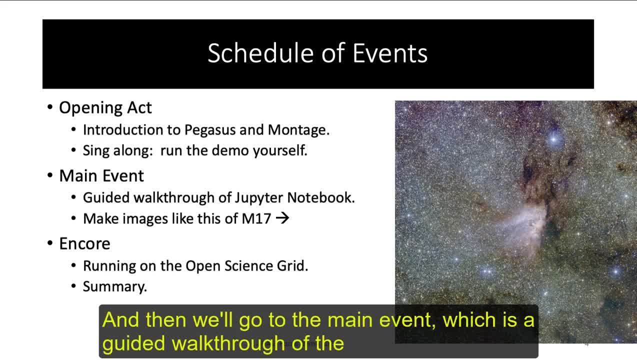 if you want to sing along with it. And then we'll go to the main event, which is a guided walkthrough: the Jupyter notebook by my colleague, John Good. It'll show you how you can make images like this one on the right-hand side, and then 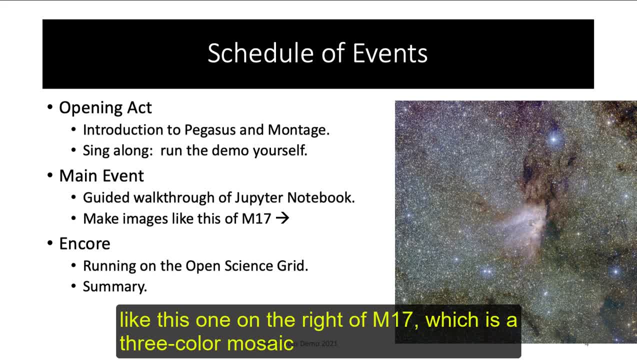 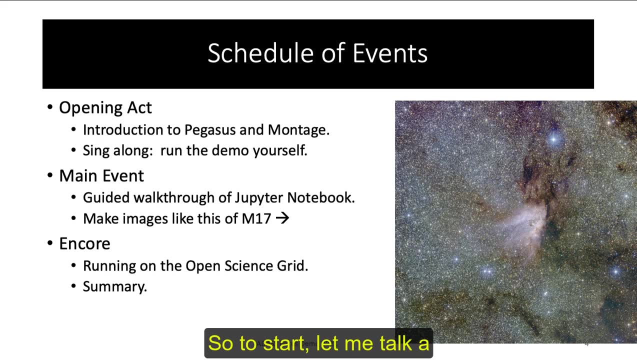 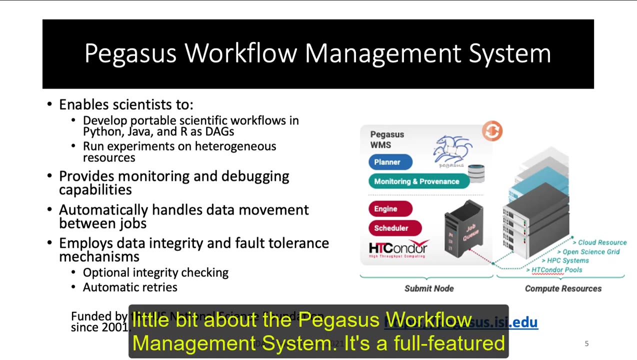 right of M17, which is a three-color mosaic made of two mass data. And finally, I'll describe what happens when we try running this on the Open Science Grid, and then I'll give you a summary of the demo. So to start, let me talk a little bit about the Pegasus Workflow Management System. 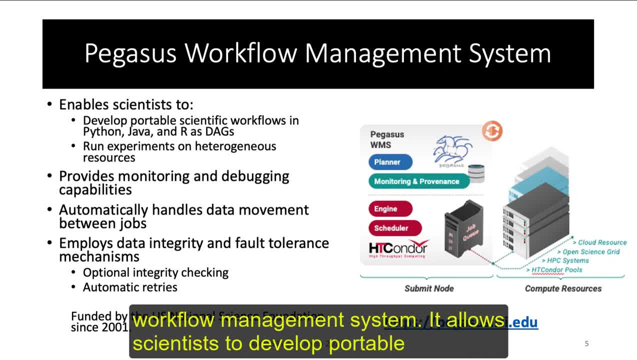 It's a fully-featured workflow management system. It allows scientists to develop portable science workflows using Python, Java or R APIs. In this case, we'll be using the Python API, And these workflows are structured as directed acyclical graphs. 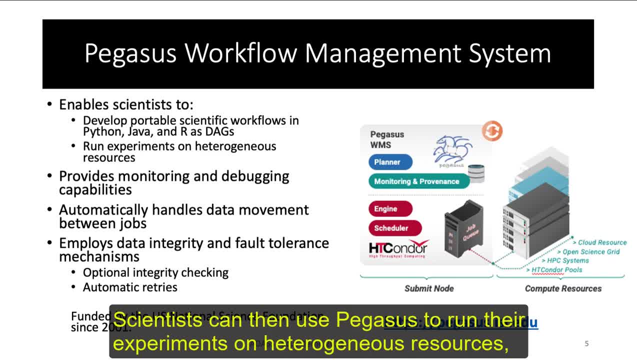 Scientists can then use Pegasus to run their experiments on heterogeneous resources, including your local machine or local cluster clouds, HPC systems, and so on. Pegasus also provides monitoring and debugging capabilities via command-line tools or, if you wish, a web dashboard. 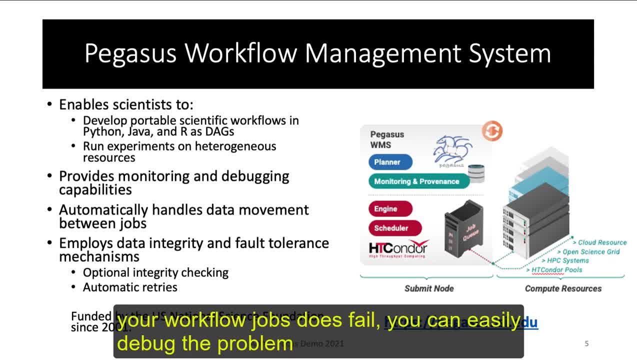 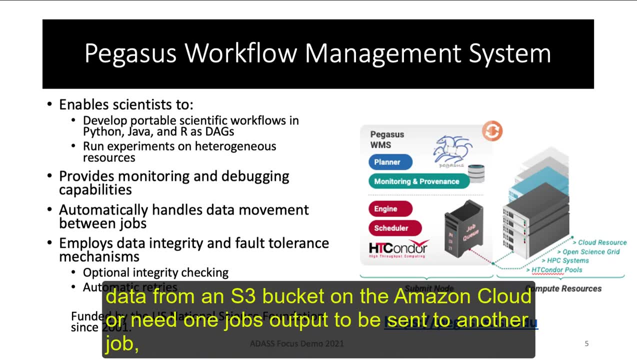 If one of your workflow jobs does fail, you can easily debug the problem with tools such as Pegasus Analyzer. Another great feature of Pegasus is that it automatically handles data movement between jobs, whether you are pulling input data from an S3 bucket on the Amazon Cloud or need one-jobs. 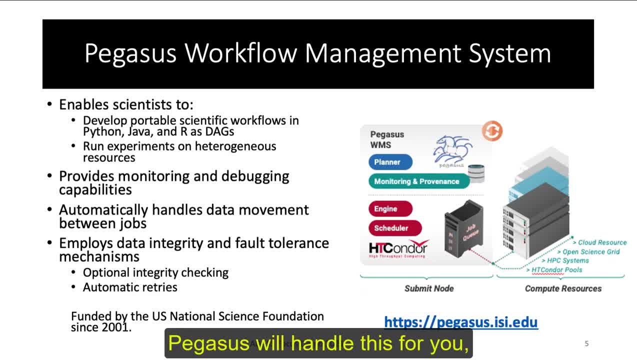 output to be sent to another job. Pegasus will handle this for you. And finally, Pegasus runs your workflows with data integrity and fault tolerance in mind. You can have Pegasus perform integrity checks on all files used in your workflow And if jobs or file transfers fail, they can be automatically rerun. 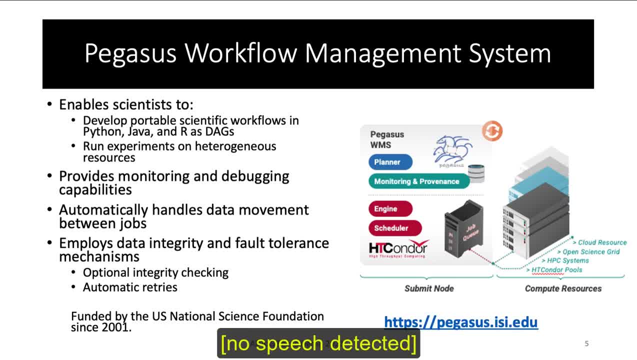 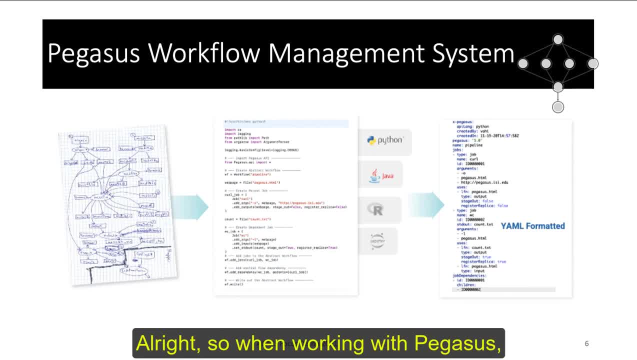 So let's take a look at the Pegasus Workflow Management System. So when working with Pegasus, you will typically have an experiment or a set of computations that need to be performed, and at a high level. it will generally look like the drawing on: 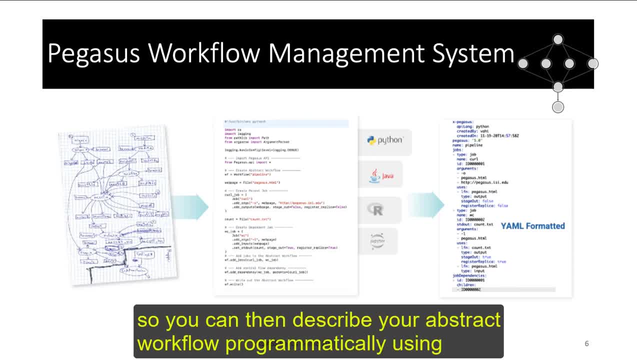 the left, So you can then describe your abstract workflow programmatically using one of the APIs, in this case Python, as shown in the center image, and once that's done, your workflow will be serialized to a YAML representation, And that's it. 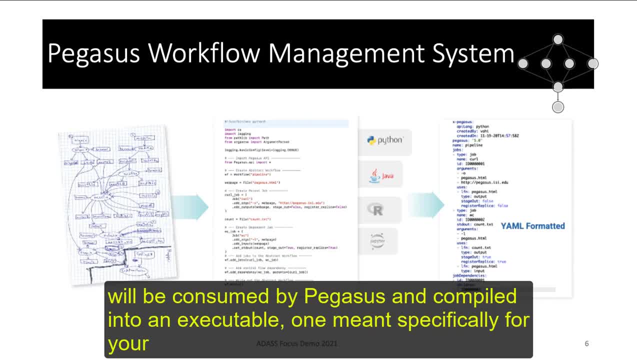 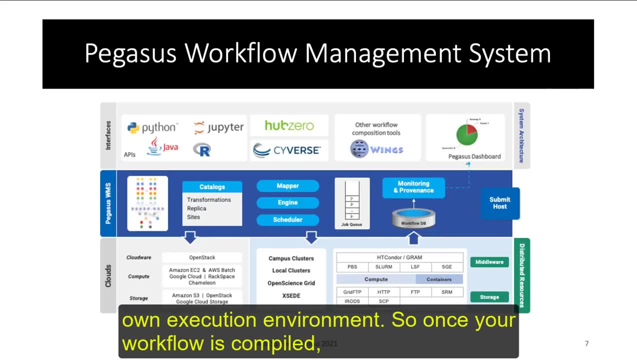 So once your workflow is compiled, it's ready to run. So at the bottom row on this chart shows some of the most common execution environments where users can run their workflows and includes cloud resources such as AWS or the Google Cloud, HPC resources such as XSeed or local clusters. 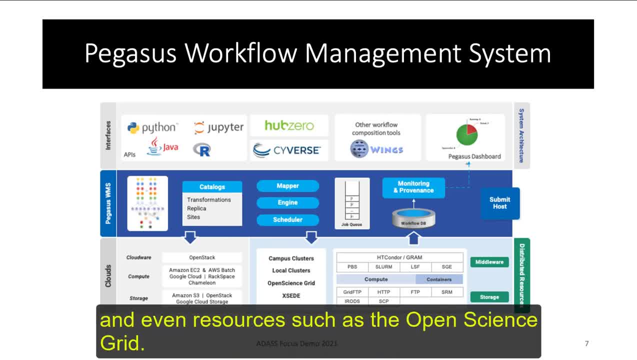 And then you can see that there are a number of different workflows that can be used to run your workflow, And I just want to mention that in the top right corner there are many different ways to run your workflow, So you can find out what your workflow should be. 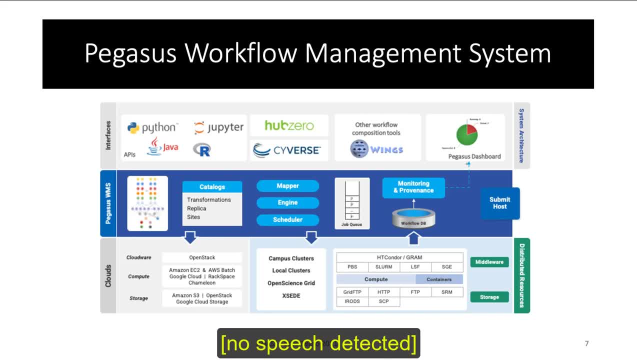 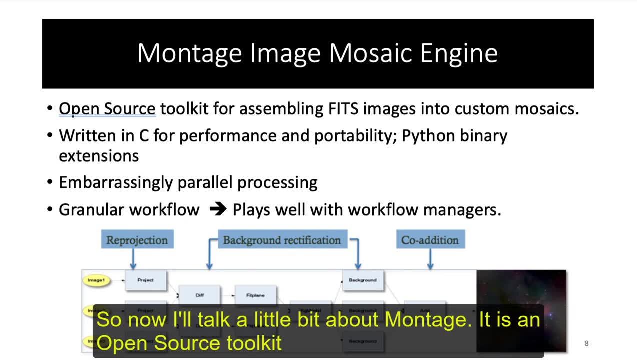 And if you've got a couple of different tools you can use, and even resources such as the Open Science Grid. So now I'll talk a little bit about Montage. It is an open source toolkit for assembling FITS images into custom mosaics. 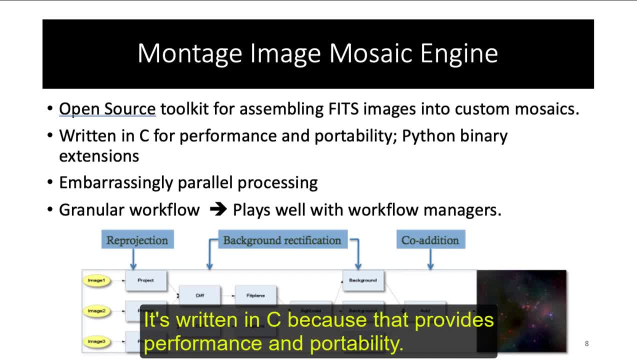 It's written in C because that provides performance and portability. We have deployed Python binary extensions of these C++, So this is really just a code that you use as a software. It's a very useful tool: routines so that you can get compiled performance in a Python environment, and 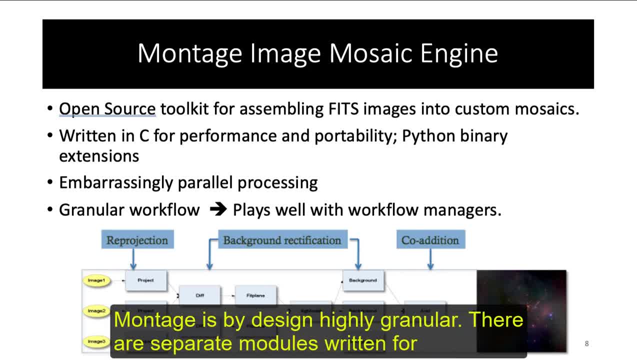 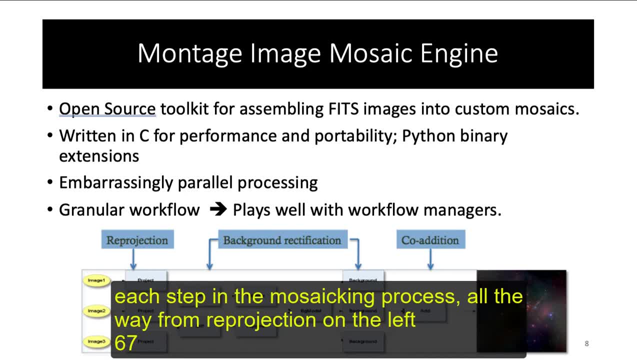 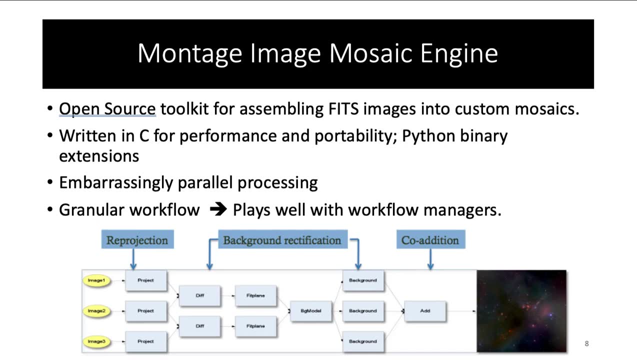 the workflow montages is, by design, highly granular. there are separate modules written for each step in the mosaicing process, all the way from reprojection on the left and the chart on the bottom to co-edition at the right and in the middle you have the background, rectification steps, background. 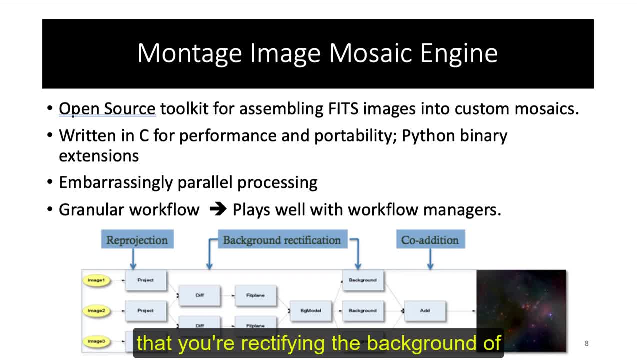 rectification simply means that you're rectifying the background of each of the images to a common level. in addition, this processing paradigm is is embarrassingly parallel. you can process each of the images that you input into your workflow on set on independent machines. we can use as many as these as 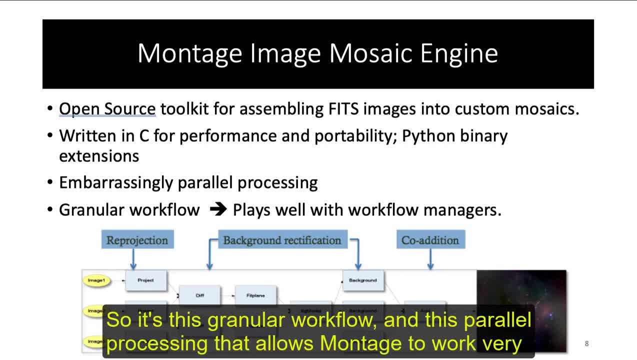 you wish. so it's this granular workflow and this parallel processing that allows montage to work very well with workflow managers, and in fact we have used montage with Pegasus before. for example, we built a 15 wavelength Atlas of the plane of our galaxy in the 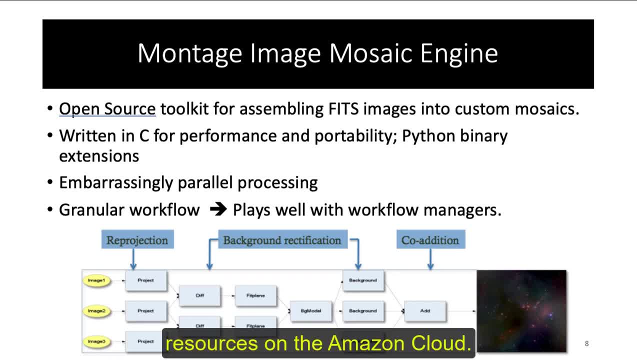 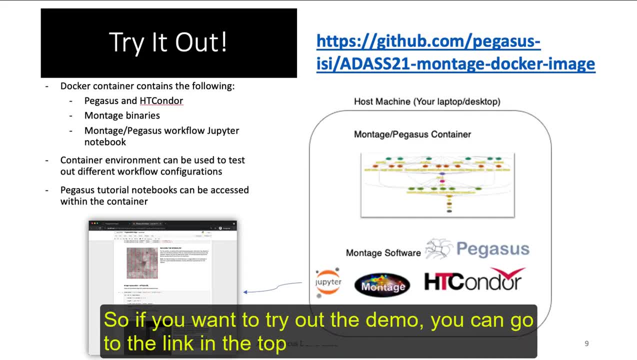 infrared using purely resources on the Amazon cloud. so if you want to try out the demo, you can go to the link in the top right hand corner of this chart. we created a docker image with everything you need to run the montage workflow Jupyter notebook. the docker image contains an installation of 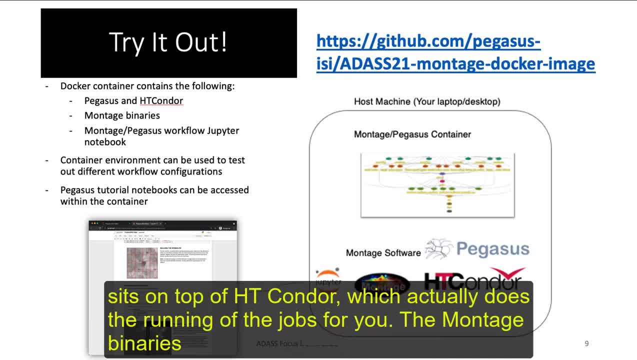 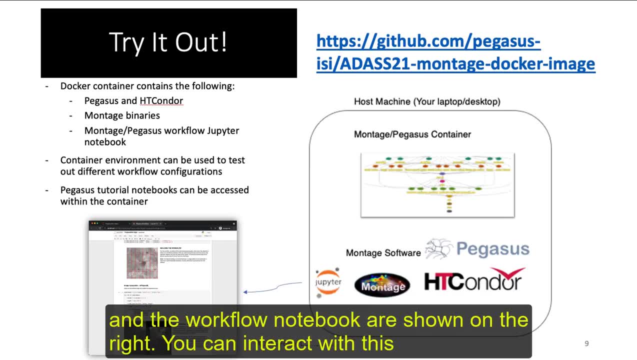 Pegasus and HT Condor. Pegasus sits on top of HT Condor, which actually does the running of the jobs for you: the montage binaries and the workflow notebook now shown on the right. you can interact with this container through Jupyter notebooks via the browser. you can even use this container environment to test out different 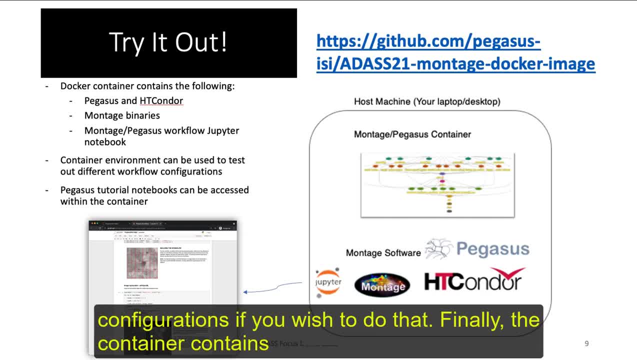 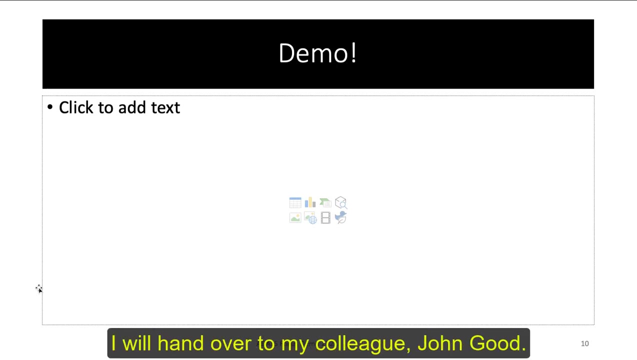 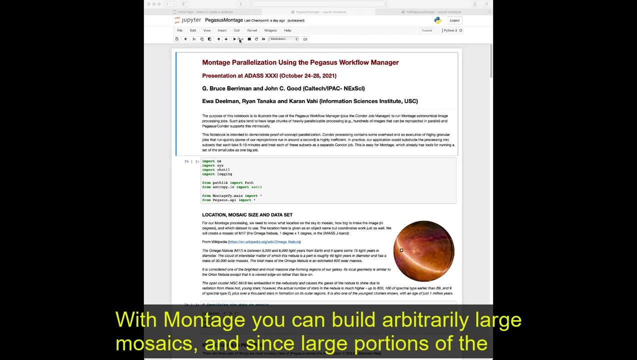 workflow configurations, if you wish to do that. finally, the container contains Pegasus tutorial notebooks if you want to learn more about how to develop your own Pegasus workflows for different applications. and now let's begin the demo I will hand over to my colleague, John good. with montage, you can build arbitrarily large mosaics and, since large portions of 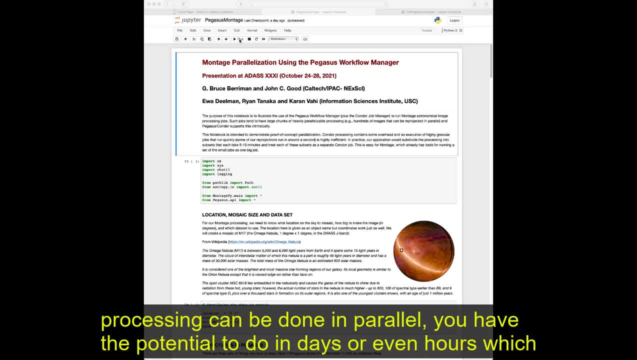 the processing can be done in parallel. you have the potential to do in days or even hours what might otherwise take six months. using cloud or cluster resources, it is now feasible to marshal tens or even hundreds of compute instances and tens of terabytes of storage for short enough periods of time that the overall 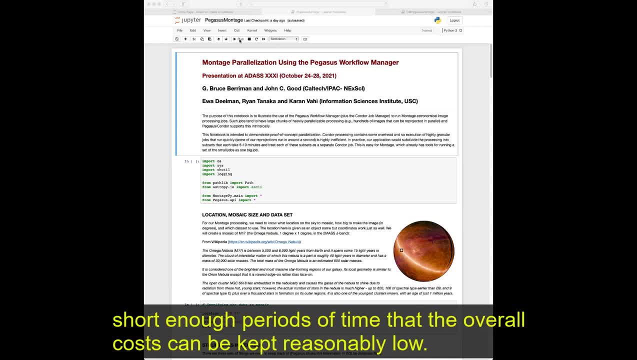 cost can be kept reasonably low, but effectively using these resources can be a major task in itself, and building an infrastructure that can effectively switch between platforms even more so. that's where Pegasus and HT Condor come in, as we shall show here. it is straightforward to explain to Pegasus. 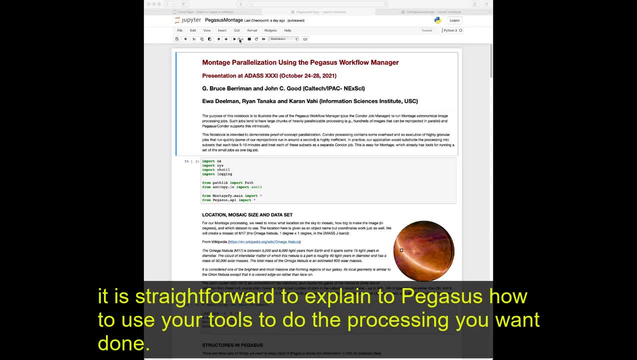 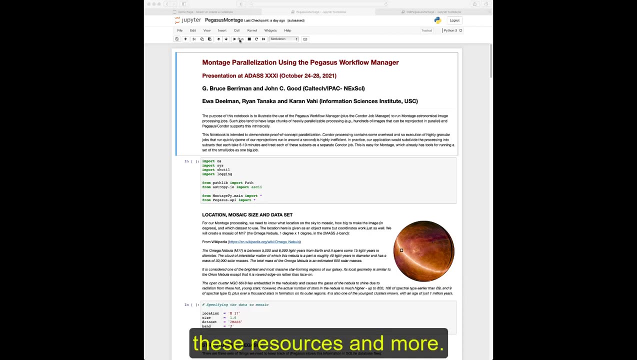 how to use your tools to do the processing you want done. then Pegasus will work out an optimal processing plan in the form of a simple and detailed that can be handed off to HD Condor. HD Condor already knows how to run such plans efficiently. on all these resources and more, All we need for plan building. 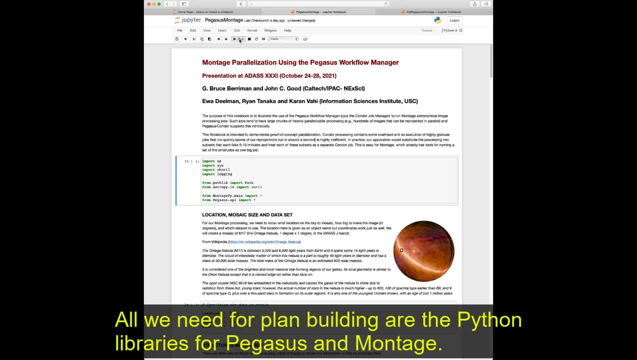 are the Python libraries for Pegasus and Montage. Montage is used here just to gather metadata about the actual data needed for the mosaic. When HD Condor runs, it will use a separate copy of Montage on the compute resource in the form of a set of Linux executables. The free parameters for the mosaic are the: 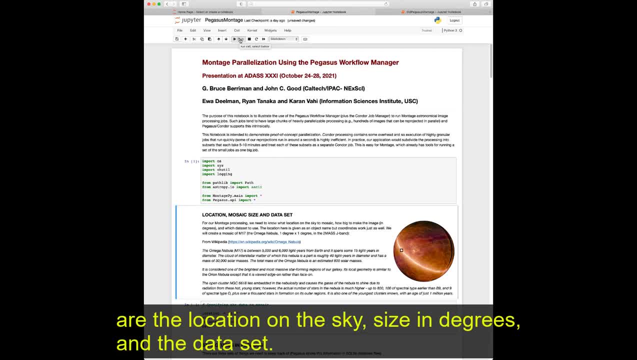 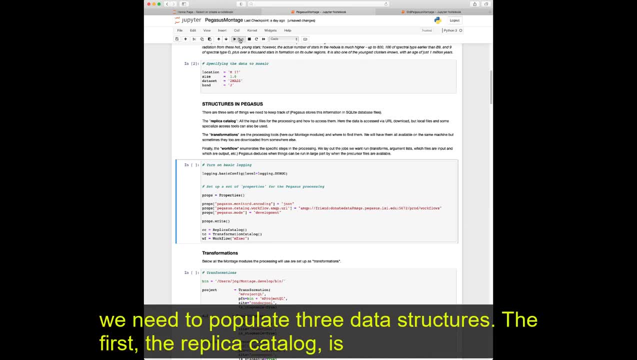 location on the sky, size in degrees and the data set. For Pegasus to do its work, we need to populate three data structures. The first, the replica catalog, is information on the files that will be needed as input, where they are. 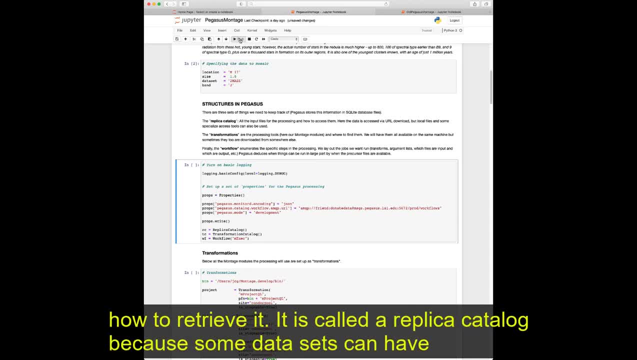 and how to retrieve them. The second, the replica catalog, is information on the files that will be needed as input, where they are and how to retrieve them. It is called a replica catalog because some data sets can have multiple available copies of the files and Pegasus can improve throughput by 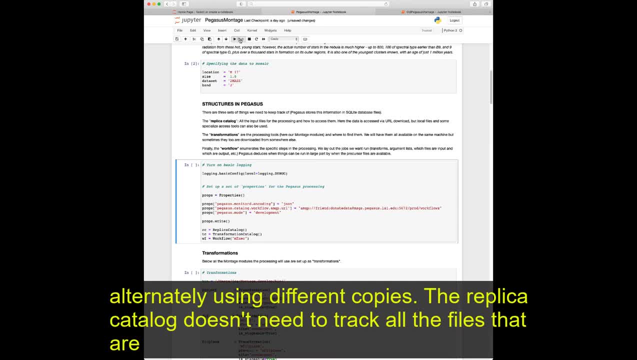 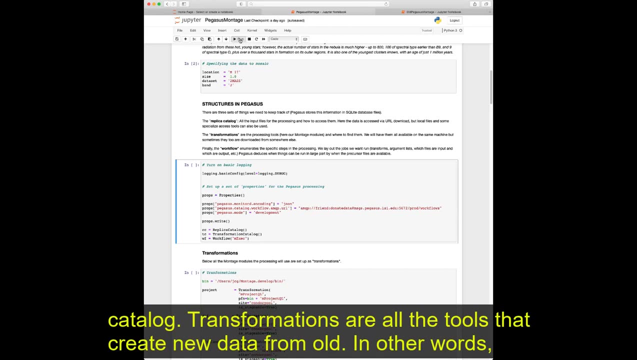 alternately using different copies. The replica catalog doesn't need to track all the files that are created during the processing. Pegasus will handle those. The second structure is the transformations catalog. Transformations are all the tools that create new data from old, in other words, the Montage. 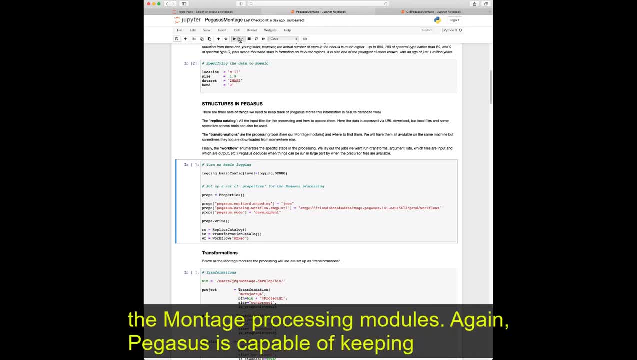 processing modules. Again, Pegasus is capable of keeping track of multiple copies of these tools, though in a case like this, they will just be executables in our local path. Finally, we have the workflow catalog, which keeps track of all the processing steps we define, the transformations used and the 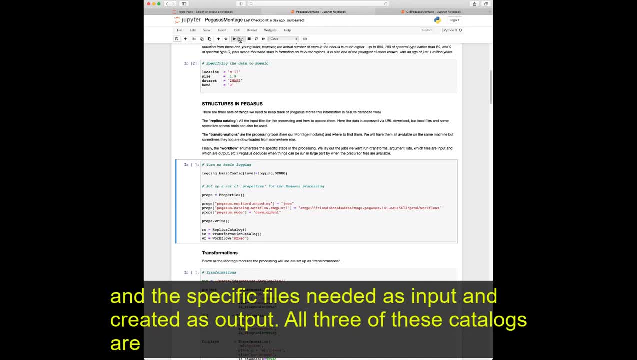 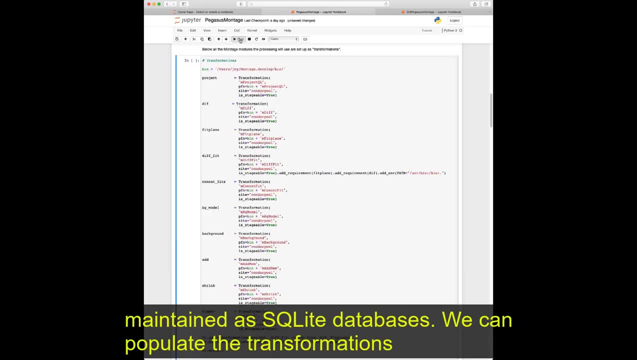 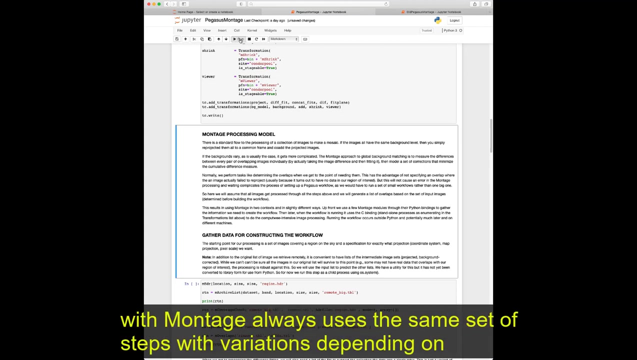 specific files needed as input and created as output. All three of these catalogs are maintained as SQLite databases. We can populate the transformations catalog up front simply by adding the paths to all the montage modules. we will use General flow for building a mosaic with. montage always uses the same set of steps with variations. 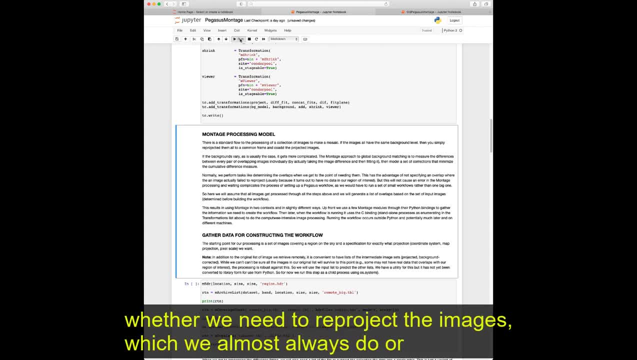 depending on whether we need to re-project the images, which we almost always do, or correct the background levels. Even for properly flux-calibrated images, backgrounds can vary, especially in the infrared. The background there depends so much on where you are in the zodiacal dust cloud and what 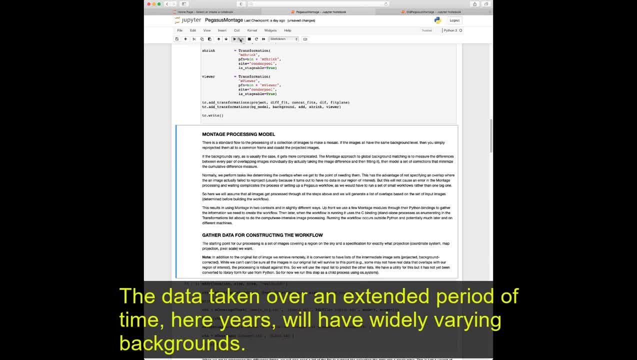 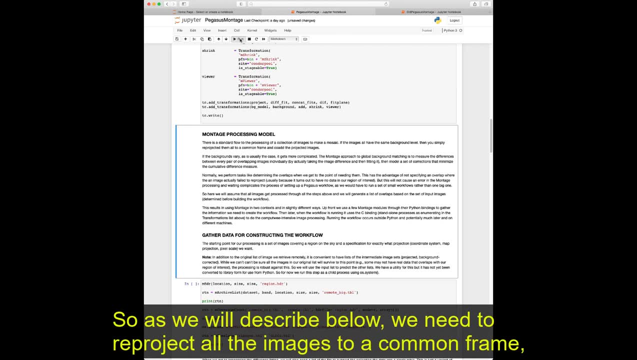 direction. you are looking that data taken over an extended period of time here years will have widely varying backgrounds. So, as we will describe below, we need to re-project all the images to a common frame, examine all the image-to-image overlaps to gather information on background differences model. 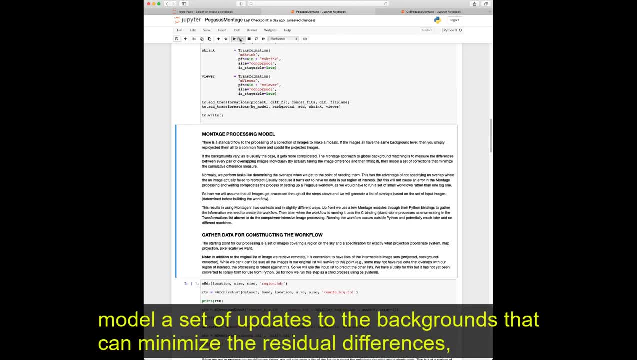 a set of updates to the backgrounds that can minimize the residual differences. apply these updates And co-add for a final mosaic. Our first steps are to define the WCS header for the mosaic we want to build and to search a remote metadata service to get a list of images we will need. 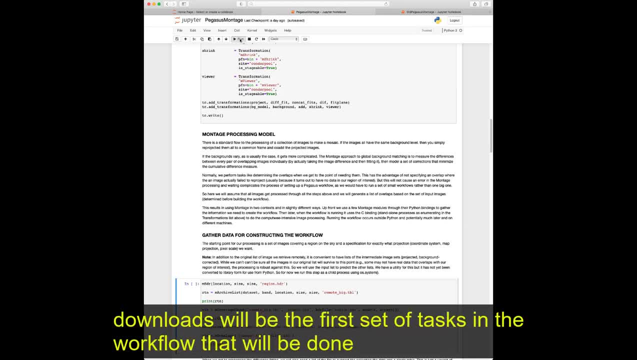 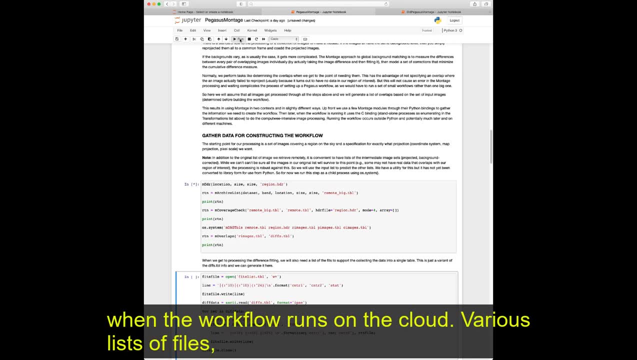 Note we are not gathering the data now. The actual data downloads will be the first set of tasks in the workflow and will be done when the workflow runs on the cloud. Various lists of files, The original data, Projected images, Reference images. 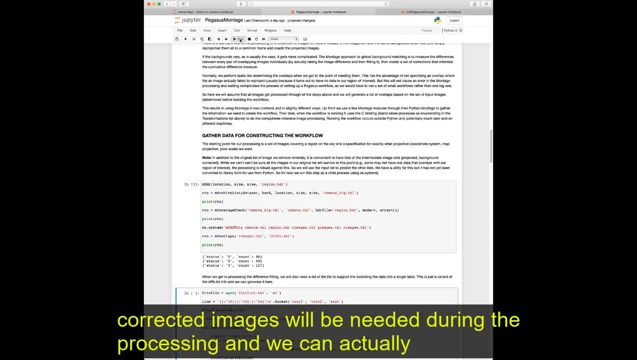 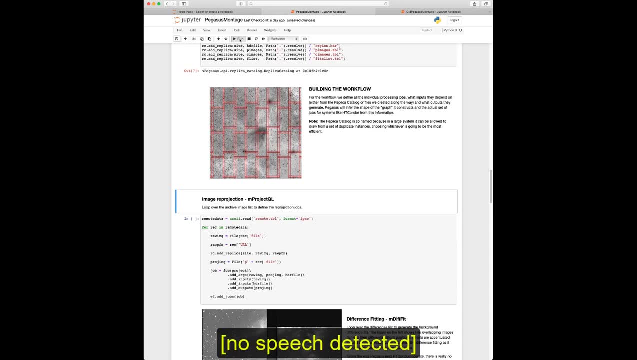 Background. corrected images Will all be needed during the processing and we can actually predict what these will be now, So we can finally start building the workflow catalog. All the images listed in the original raw data table need to be added to the replica catalog. 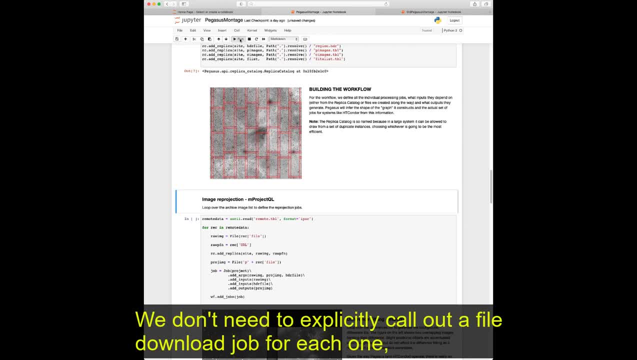 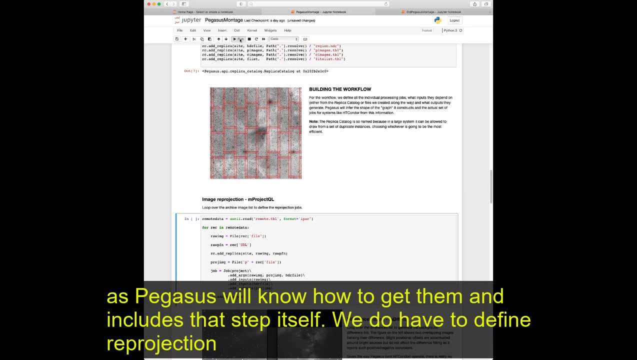 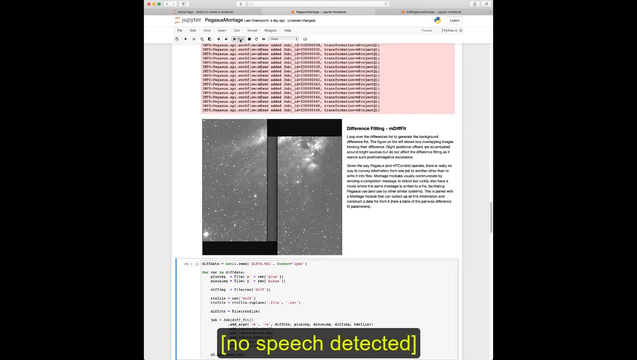 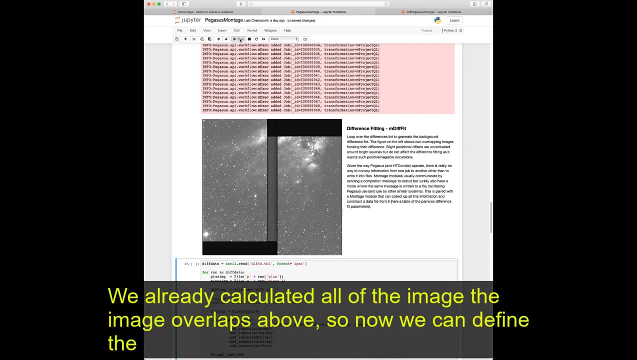 We don't need to explicitly call out a file download job for each one, as Pegasus will know how to get them. That includes that step itself. We do have to define reprojection jobs for each image. We already calculated all of the image-to-image overlaps above, so now we can define the jobs. 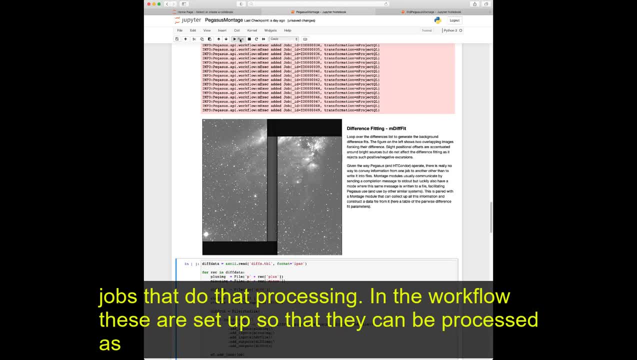 that do that processing In the workflow. these are set up so that they can be processed as soon as the reprojected images for each pair become available. The workflow is set up so that they can be processed as soon as the reprojected images. 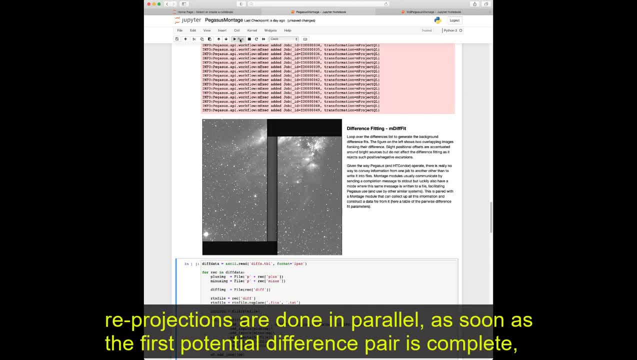 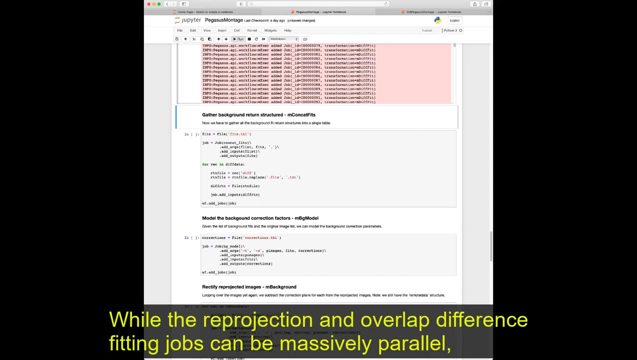 for each pair become available. So in the extreme case where all the reprojections are done in parallel, as soon as the first potential difference pair complete, the difference job will start, While the reprojection and overlap difference fitting jobs can be massively parallel. the 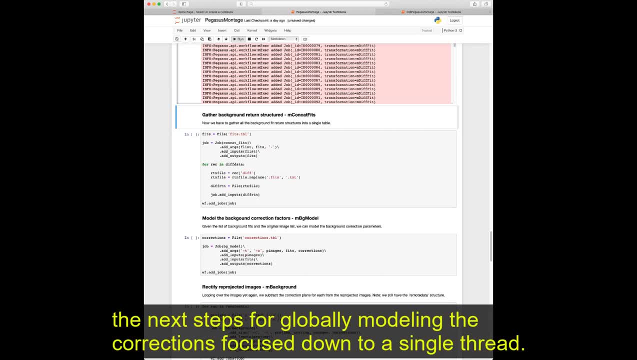 next steps for globally modeling, the corrections focus down to a single thread. First we combine all of the individual difference fits into a single table. Then we run the modeling code. This program iteratively estimates corrections for all the images and is optimized to be. 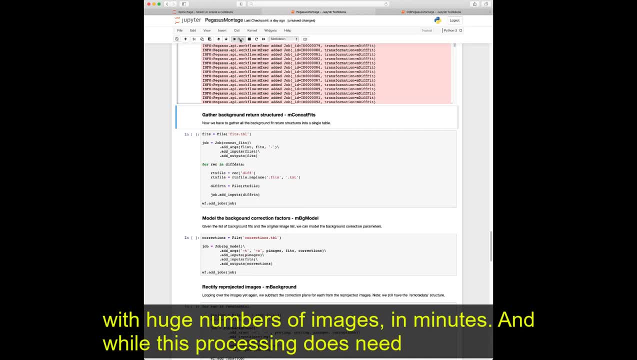 able to do this even with huge numbers of images in minutes, While this processing does need to wait until all the reprojections and difference fittings are complete. those steps are fairly uniform in processing time, so will all tend to finish at about the same time. 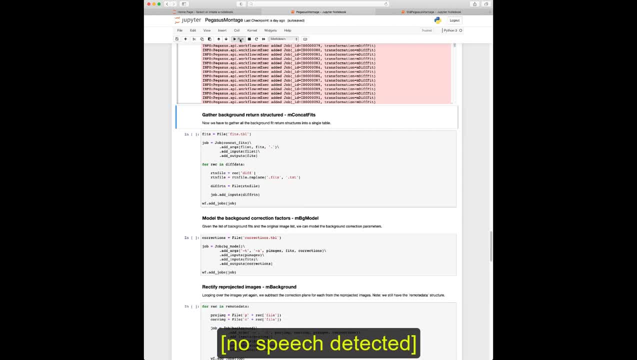 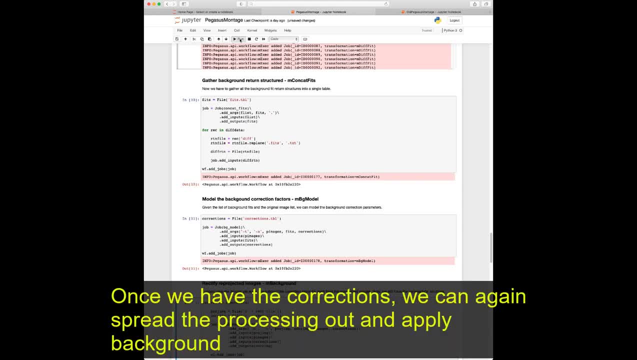 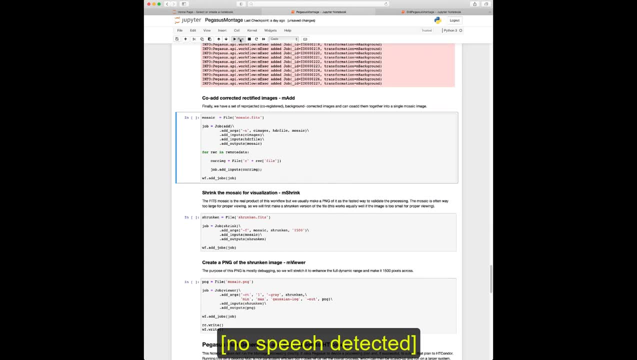 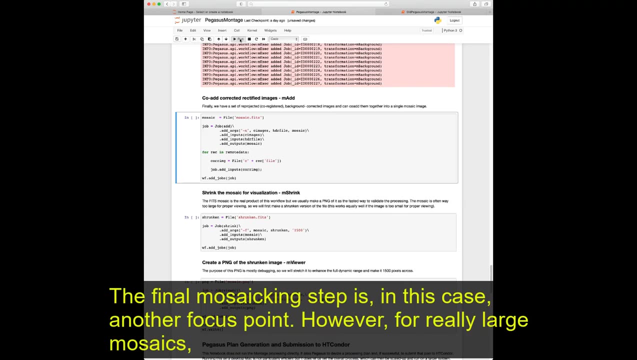 Once we have the corrections, we can again spread the processing out and apply a background correction in parallel. The final mosaicing step is, in this case, another focus point. However, for really large mosaics, we often find that in practice we prefer to co-add. 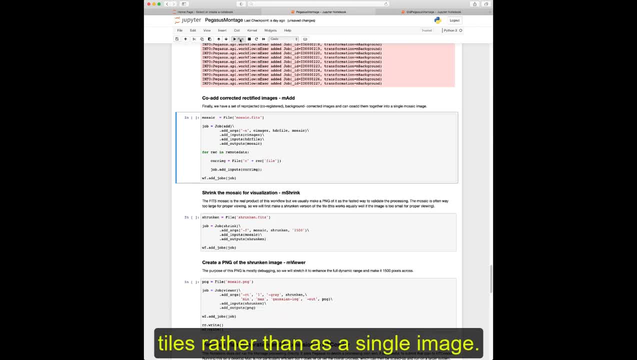 as a regular set of tiles rather than as a single image. The final mosaicing step is, in this case, another focus point. However, for really large mosaics, we often find that in practice, we prefer to co-add as a regular set of tiles rather than as a single image. The final mosaicing step is, in this case, another focus point. However, for really large mosaics, we often find that in practice, we prefer to co-add as a regular set of tiles rather than as a single image. The final mosaicing step is, in this case, another focus point. However, for really large mosaics, we often find that, in practice, we prefer to co-add as a regular set of tiles rather than as a single image. The final mosaicing step is, in this case, another focus point. However, for really large mosaics, we often find that, in practice, we prefer to co-add as a regular set of tiles rather than as a single image. 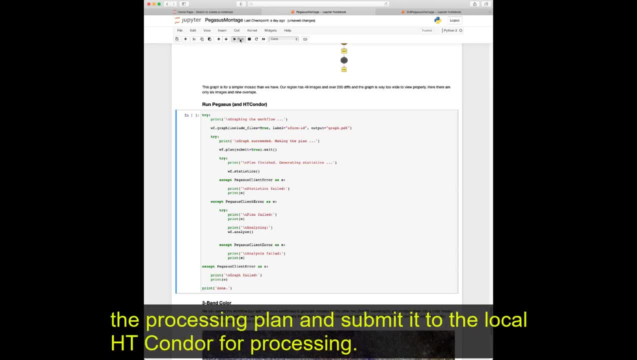 That means we want Pegasus to make the processing plan and submit it to local hdCondor for processing. That means we want Pegasus to make the processing plan and submit it to local hdCondor for processing. We also want it to wait for hdCondor to finish. 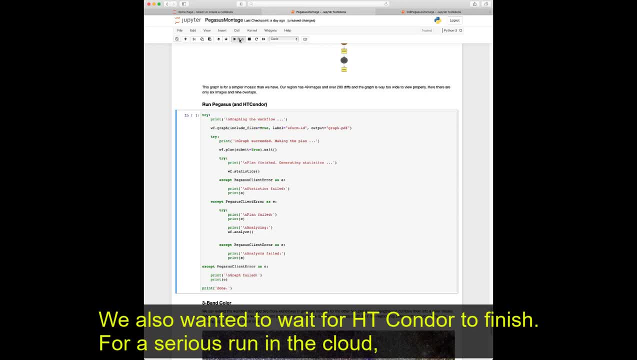 We also want it to wait for hdCondor to finish For a serious run in the cloud. we would decouple all this building the plan and then later submitting it to hdCondor on the cloud to run in background. Here, Pegasus will monitor the hdCondor run and report progress in real time. 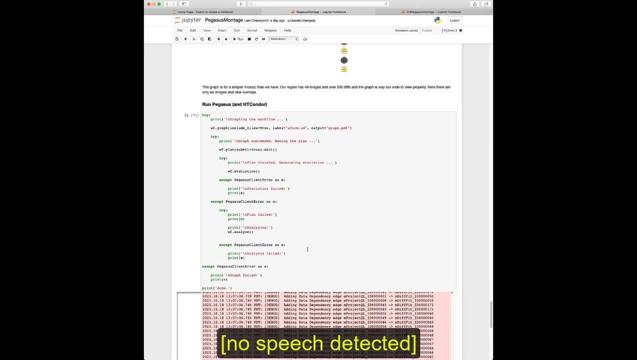 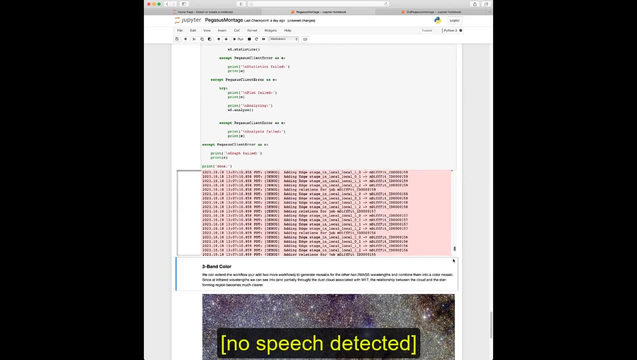 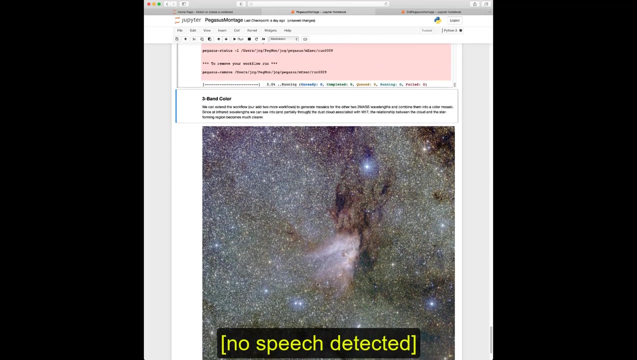 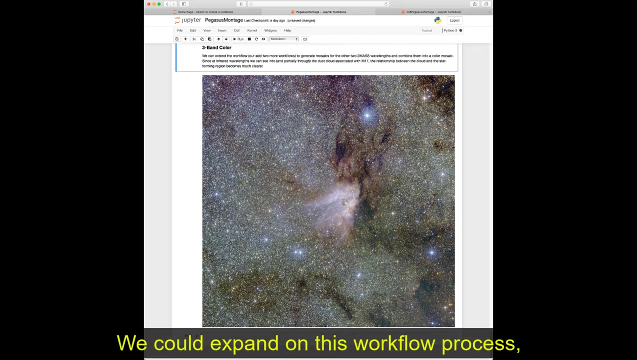 We won't wait for that to finish. Thank you. We could expand on this workflow to process all three bands needed to make a color composite at the end, or, more likely, would submit the processing as three workflows. We've done that here and made this composite. 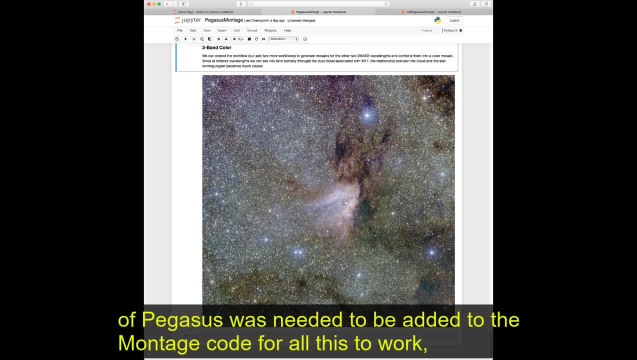 It's important to note that no knowledge of Pegasus needed to be added to the montage code for all this to work. That is generally true for Pegasus processing. It is true that for typical montage processing, when one would capture and analyze the response messages from the montage modules to control the flow. 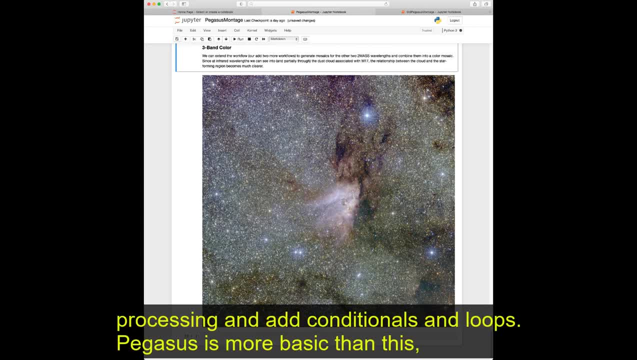 this allows you to react to the processing and add conditionals and loops. Pegasus is more basic than this. It only checks the program return statuses and for the existence of expected output files, And this is a mode that works fine for well-defined pipelines of the sort described here. 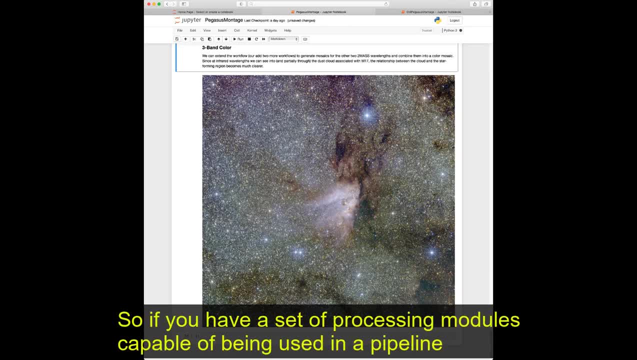 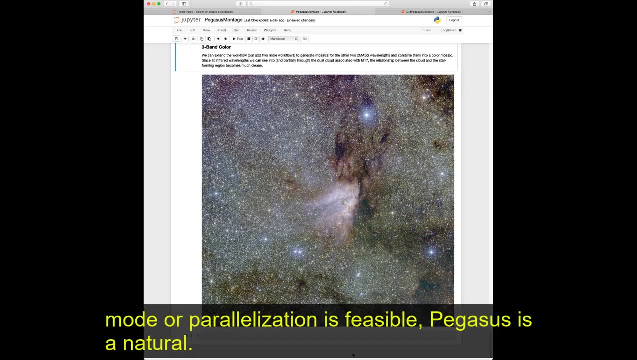 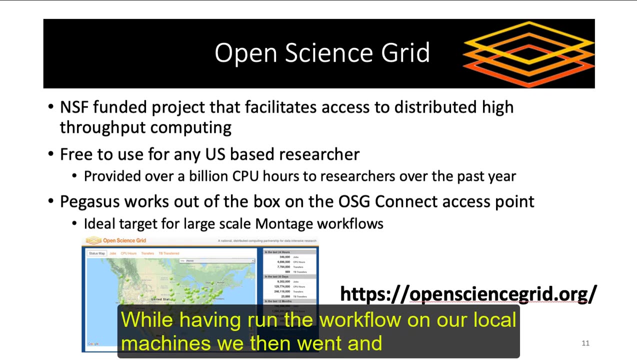 So if you have a set of processing modules capable of being used in a pipeline mode, or parallelization is feasible. Pegasus is a natural Well. having run the workflow on our local machines, we then went and ran it on the OpenScience grid. 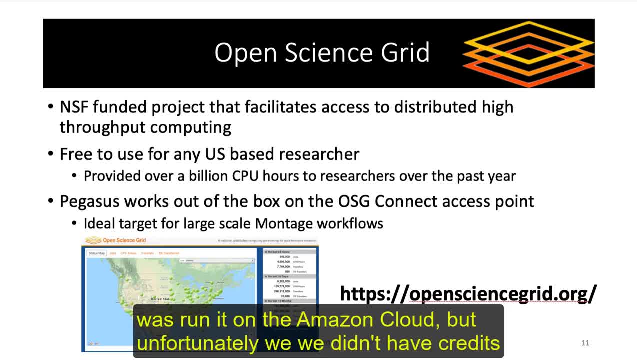 Now, what we really wanted to do was run it on the Amazon cloud, but unfortunately we didn't have credits left, so we were not able to do that. The OSG is a good choice. It's a parallel platform, because Pegasus works out of the box on the OSG connect access point. 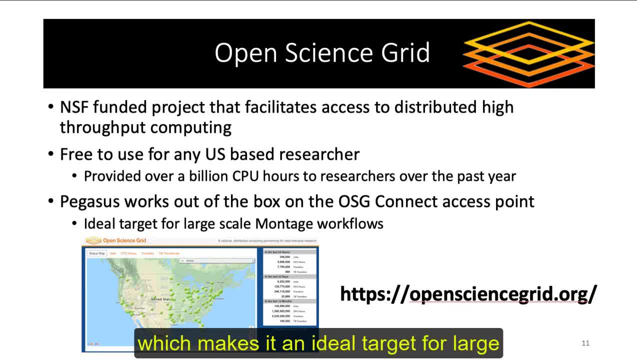 We know this already, which makes it an ideal target for large workflows such as those provided by Montage. The OpenScience grid itself, or OSG as it's now known, is an NSF-funded project that facilitates access to high-throughput computing. 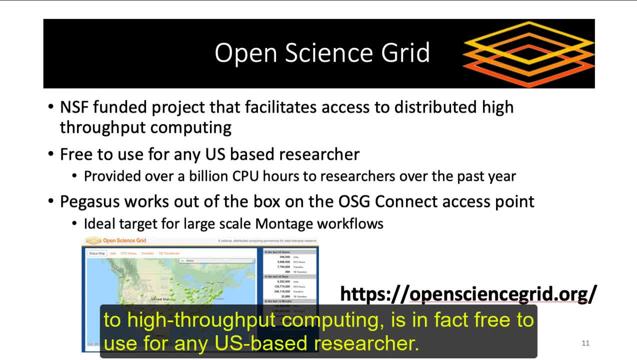 It is, in fact, free to use for any US-based researcher and indeed, in the past year it's provided over a billion CPU hours to researchers. All right, so what we did was we took our Montage workflow and ran it on OSG. 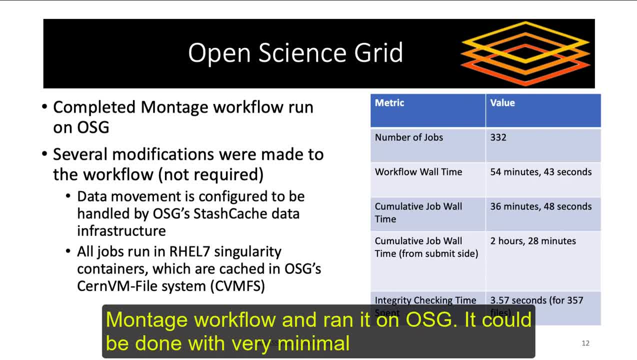 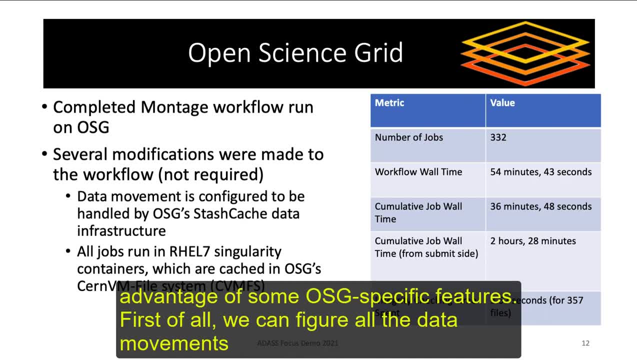 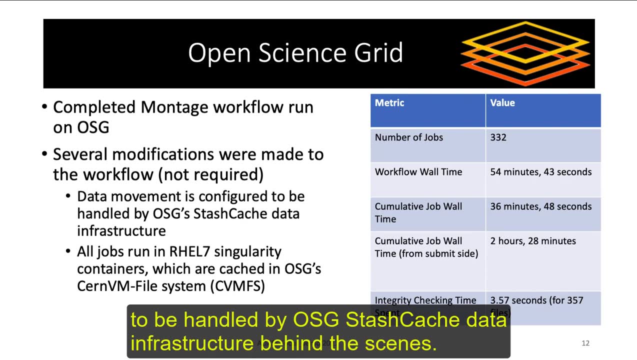 It couldn't be done with very minimal modifications to the Python workflow script. We did make several changes to take advantage of some OSG-specific features. Well, first of all, we configured all the data movements to be handled by OSG stash cache data infrastructure. 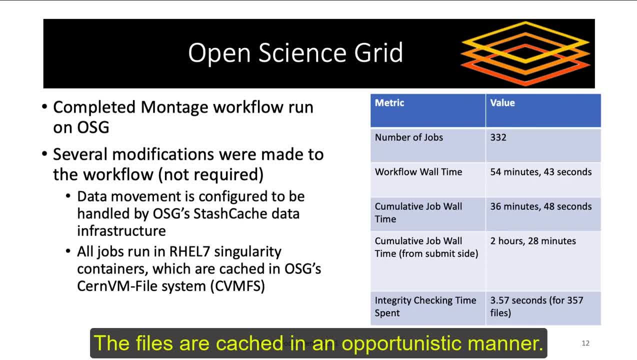 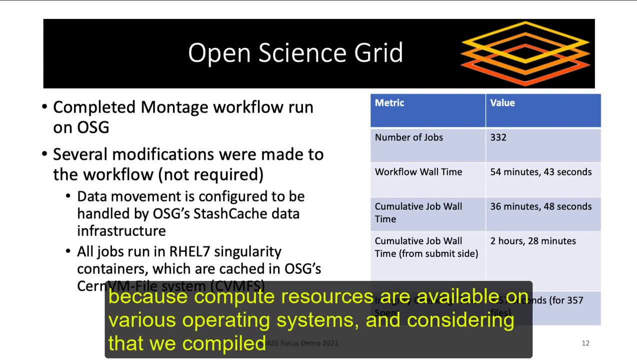 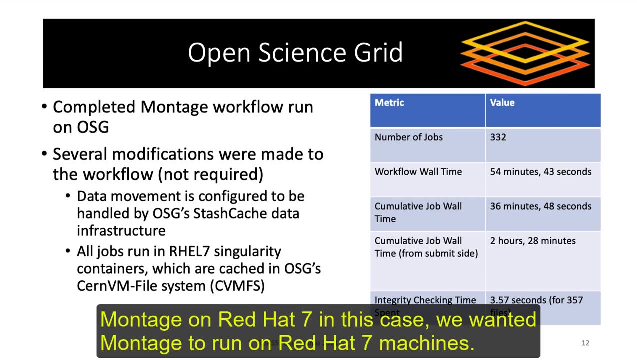 Behind the scenes, the files are cached in an opportunistic manner that requires no extra effort on our part. Second, because compute resources are various operating systems and considering that we compiled Montage on Red Hat 7, in this case we wanted Montage to run on Red Hat 7 machines. 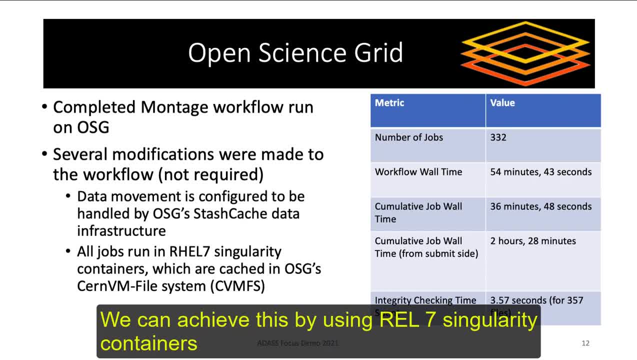 We can achieve this by using RHEL 7 singularity containers that are cached within OSG's CERN VM file system, So setting this up required us only to change a few lines in the workflow generation script. On the right-hand side we show some metrics that Pegasus reported about our run on OSG. 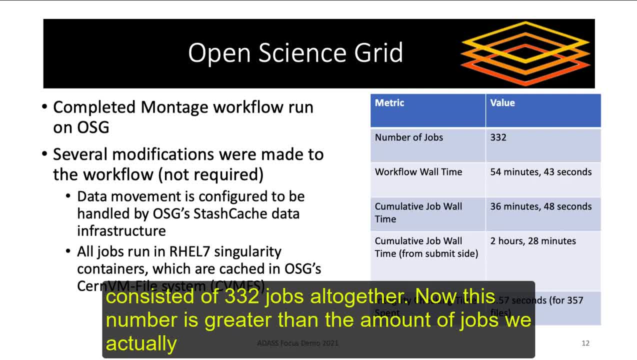 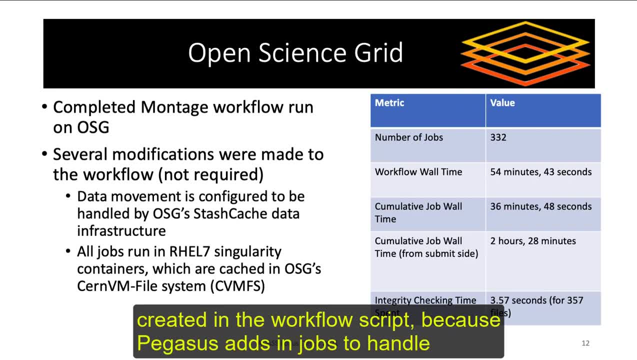 First of all, the workflow consisted of 332 jobs altogether. Now, this number's greater than the amount of jobs we actually created in the workflow script, because Pegasus adds in jobs to handle tasks such as data staging and clean-up. Next, there is the workflow wall time, which, believe it or not, is the workflow wall time.